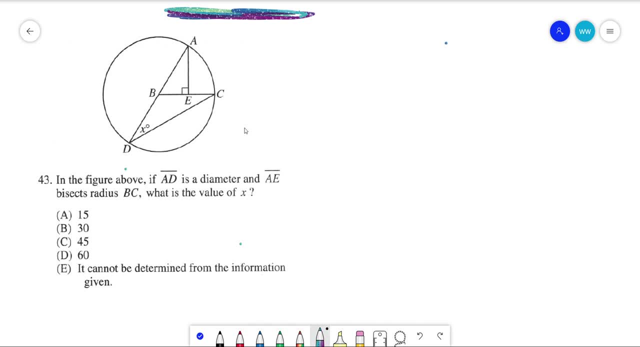 X Looks confusing, unless you know that AB is a radius and they just said that AE bisects this radius. So that means that AE cuts BC in half. So we can just call this. let's see, we could call BE. we could just call it S. Okay, so we know that BE, that S. 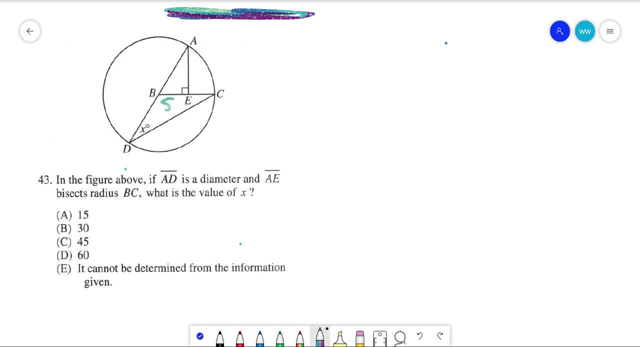 is half of the radius AB. so we call this 2S And we know we have a right triangle. I know they don't know that they're right triangles, but they're right triangles. So we know that they're right triangles. So we know that they're right triangles. So we know that they're right triangles. 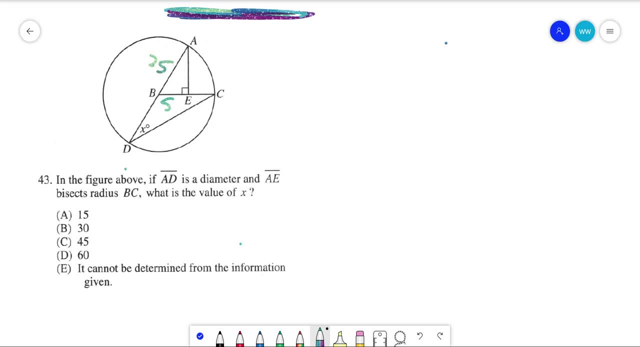 look like fives. pardon me, I should not have chosen S. Let's look, let's just call it G, Why not? Just so we don't get confused. G 2G: there we go, All right, so when you have a right triangle, 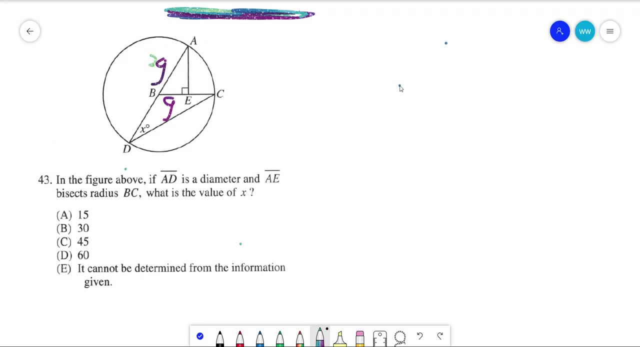 and the smallest side is half the size of the hypotenuse, which this is. then you have a 30,, 60,, 90 triangle, All right, so just keep this in mind, We know that this. so you have your 90 degree angle, anything, that's any side that's opposite the. 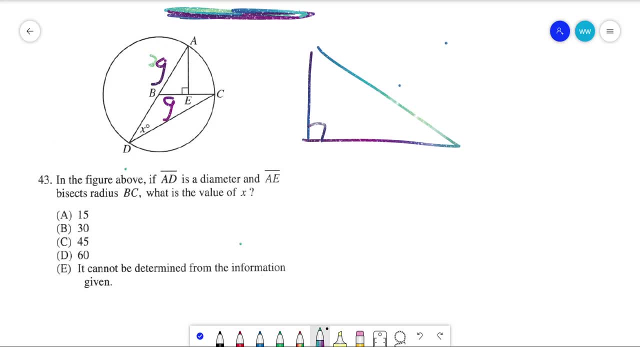 right angle is the biggest and it's the hypotenuse. So this is G, this is going to be 2G And even though this isn't particular to the problem, you should still know the full dimensional scale of a 30,, 60, 90 right triangle is what we have here, And then it's also going to be G. 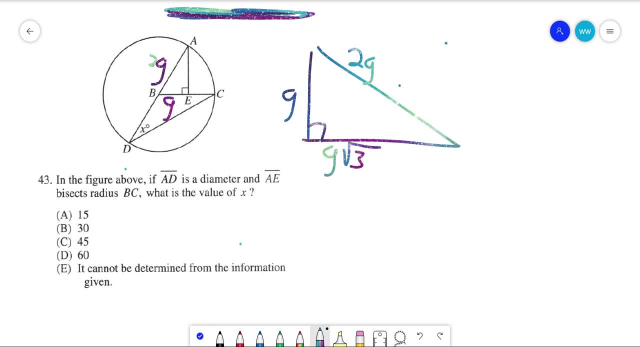 times radical three. So the second largest side is just the measure of the smallest side. times root three never fails. Okay, so we'll just say this: So this is going to be 60 degrees and this is going to be 30 degrees. All right, so 30 degrees is. 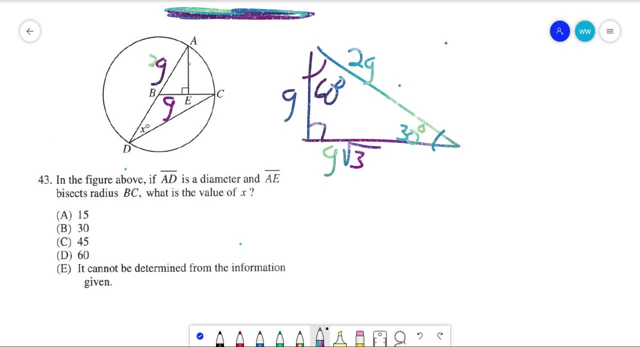 always going to be opposite the smallest side. So we know that this guy AC is 30 degrees, Oh, all right. And if we know that this side's 30,, this side's 90, then we know that this angle is 60,, 60 degrees, All right. And then that will tell us all right.